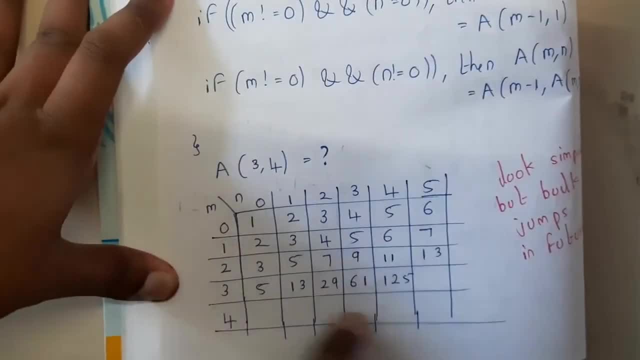 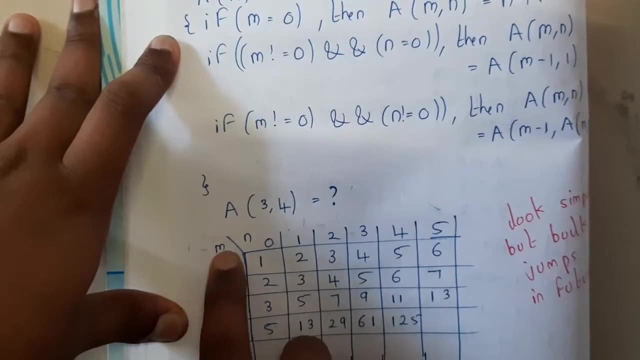 so basically the values in matrix, right? so basically 0, 1, 2, 3, 4, 0, 1, 2, 3, 4. so let us solve line by line, okay? yes, so initially the value of m is 0 for this all row, right? so the simple. 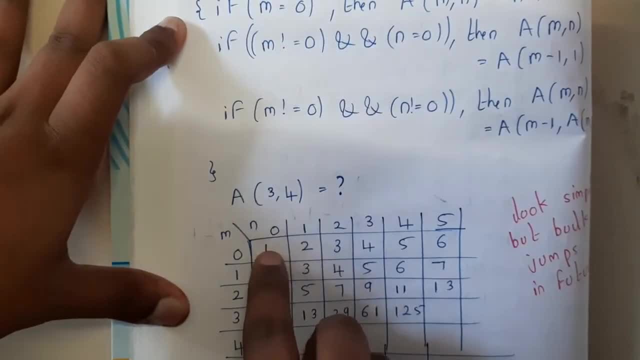 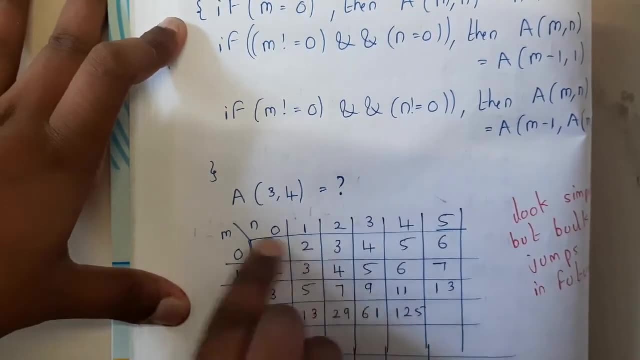 condition is nothing, but just add n plus 1. so what is 0 plus 1? it is 1. what is 1 plus 1? it is 2. what is 2 plus 1? 3, 3 plus 1, 4, 4 plus 1, 5, 5 plus 1, 6. so now we are done with the first row, luckily. 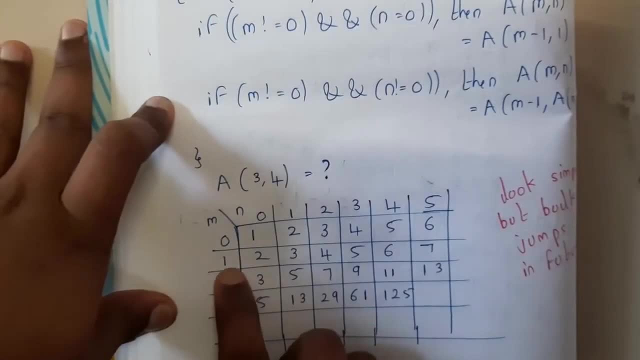 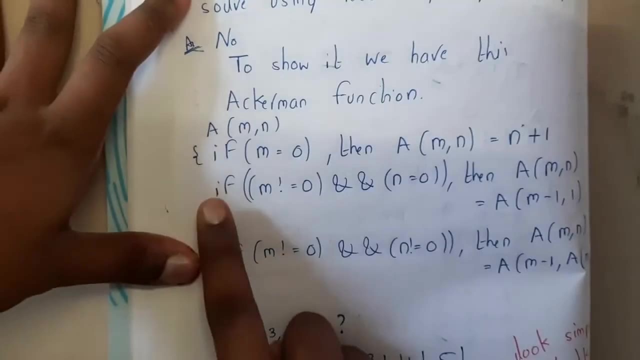 right, yes, so let us move to the second row. so in second row, m is a 1 right and n is varying from 0, 1, 2, 3. so when m is a 1, what? what are the thing we are doing? so if m is not equal to 0 and n equal, 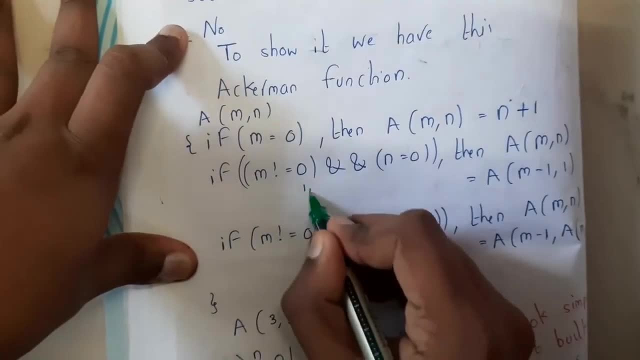 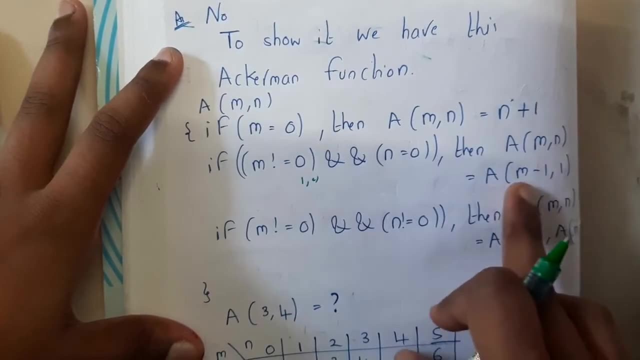 to 0. so this is the condition, right. so when 1: 1 comma 0: okay. so at this time, what we are doing is nothing. but it is nothing but equal to a of m minus 1 comma 1. so this is the condition, right. so when 1 comma 0: okay. so at this time, what we are doing is nothing. 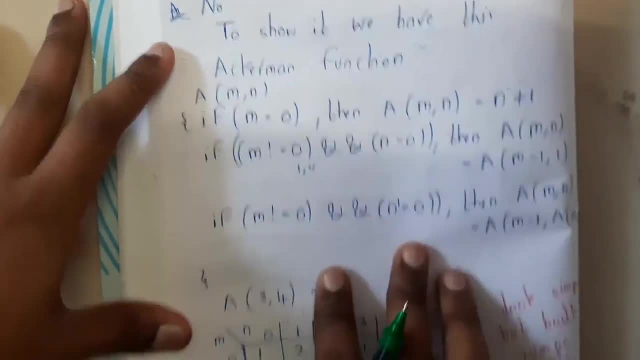 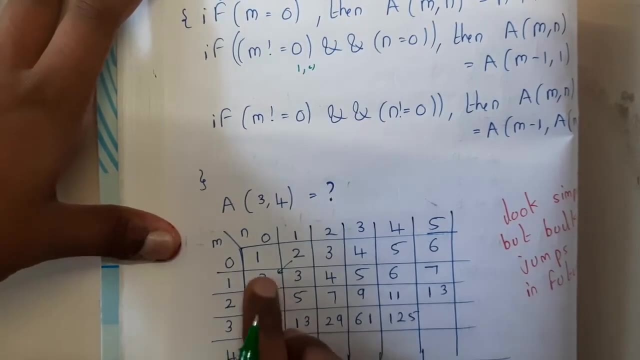 so m minus 1 is a nothing but 1 minus 1, that is 0 comma 1. so what is a 0 comma 1? that is a 2. so this value is returned here. okay, so in that way, if you keep solving, you will get all the values in. 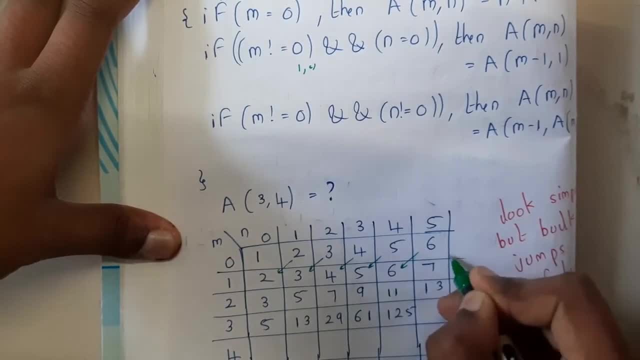 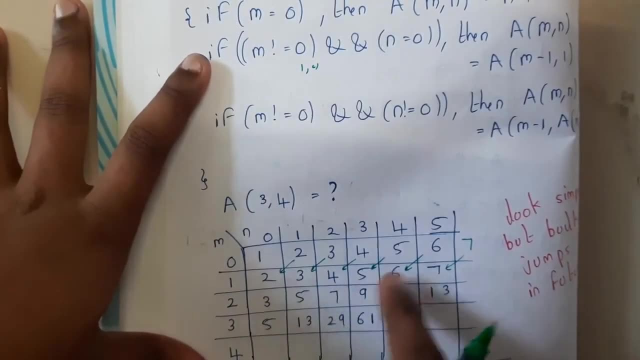 that way only. okay. so here you will be getting 7, and that 7 will be here. so once you observed this, you will be thinking that, okay, so this pattern will be followed. so 3, 4, 5, 6. but it is not true, okay, yes, so once you solve a 2, 0, 2 comma 0, so for 2 comma 0, it is a 1 comma 0 and you get a. 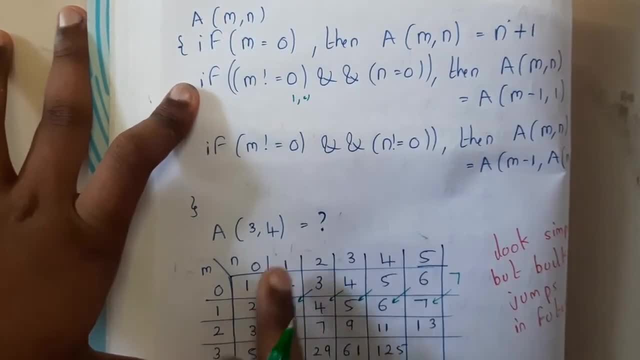 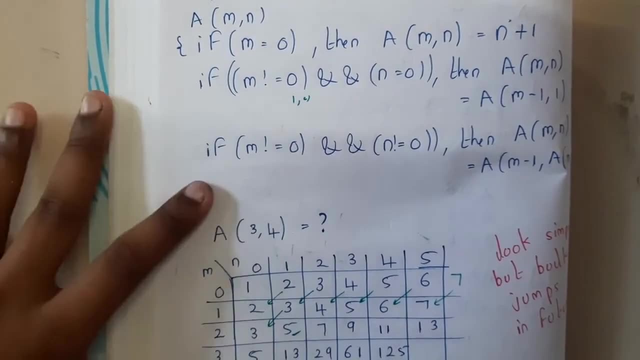 1 comma 1, so that here we got 3 value, but for 2 comma 1 you will get 5. guys, guys, please solve it. guys, because it is a bit lengthy. so if you want me to solve, i can solve for 1 or 2, okay, so let us. 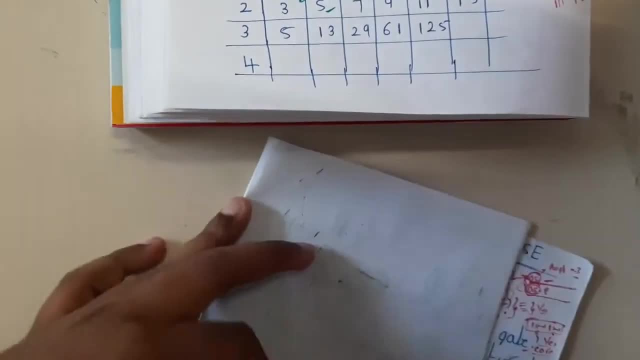 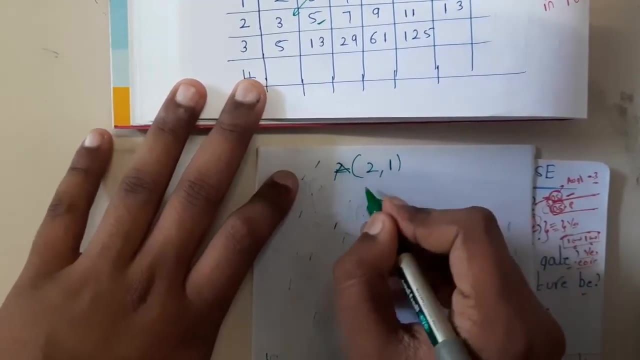 try for 2 comma 1, a of 2 comma 1, as we have some values right, so a of, sorry, a of 2 comma 1. so both of them are not equals to 0, so the result will be a of m minus 1, that is, a 1 comma a of. 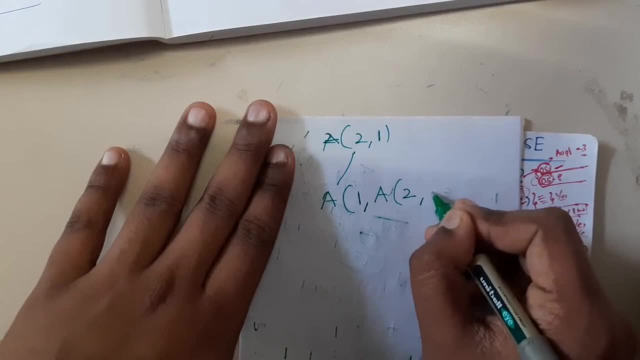 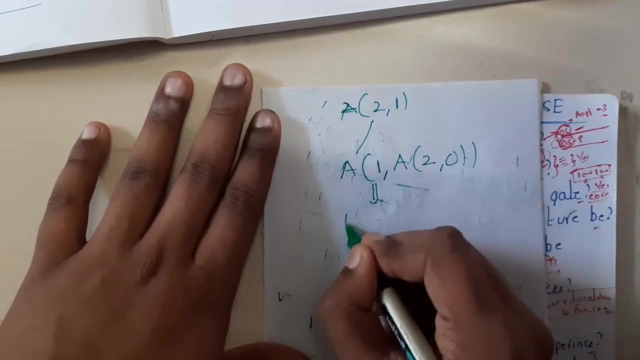 a of m. what is m? that is a 2 and what is a 0? 2 of 0, okay, so this is a nothing. but we are having a of 2 comma 0 value, right? yes, so a of 2 comma 0 value is a 3 guys. so a of 1 comma 3 is nothing. 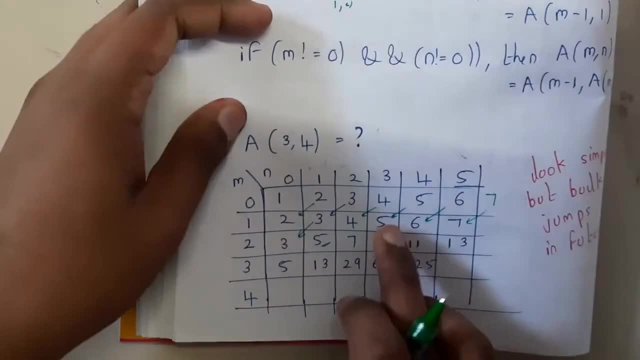 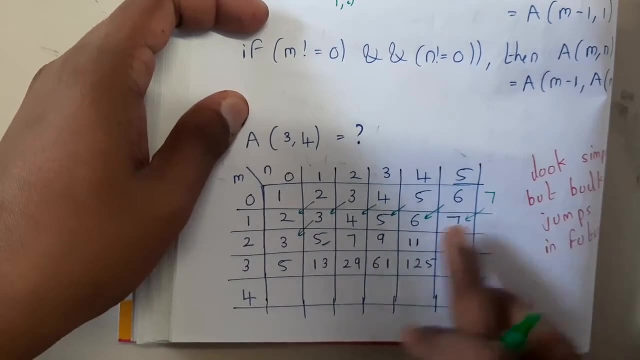 but 5. so in this way. so we got 5 here, okay. so we got this value here, okay. so again you understood the pattern. so there is one gap. so again here you will be getting 7 value, here again 9 value, 11 value, 13 value. so till now it is okay. so you are thinking that there is some pattern in it, right? 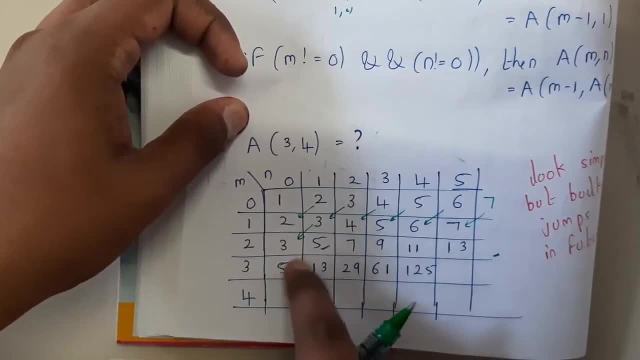 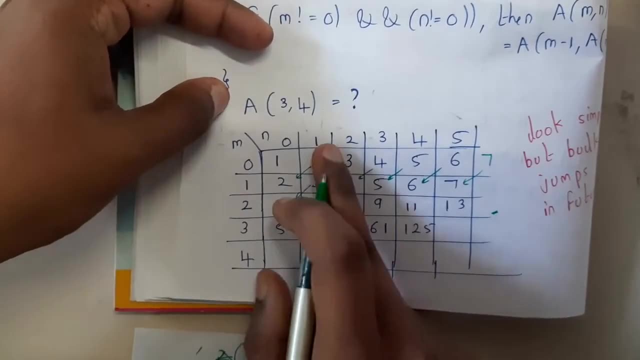 just arrows. after that we got a 1: 1 gap. again. you will think 2: 2 gap or 3: 3 gap, but when you solve for 3 comma 0, you will be getting 5. it is okay, but when you solve for 3 comma 1, it will be. 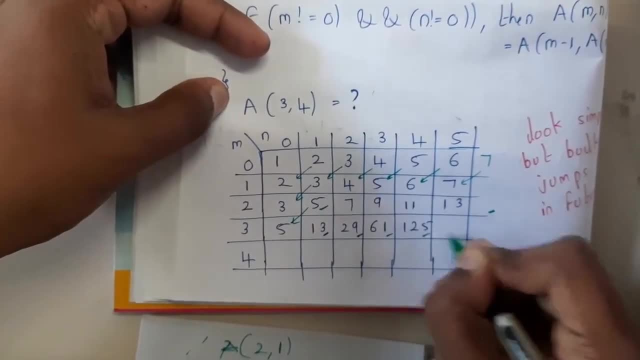 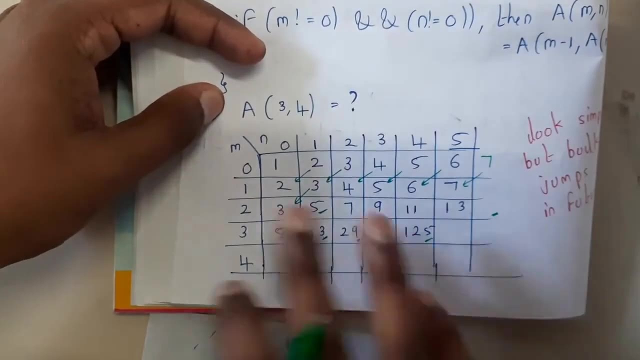 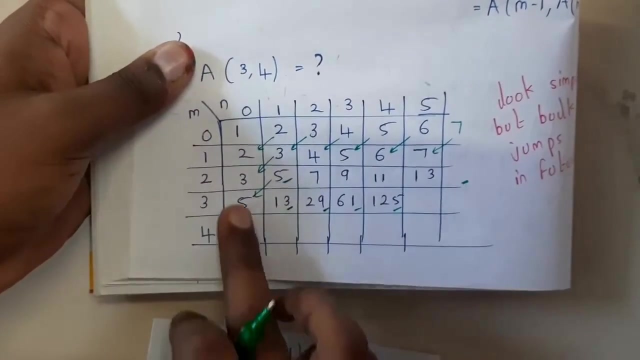 13 and after that 3, comma 2, it will be 29. so, even though you think there is a pattern, but there is no pattern, guys. so each line is independent using this formula. so that is what we can showcase using this concept of eckerman function guys. okay, yes, so it looks really simple, but it jumps, the jumps. 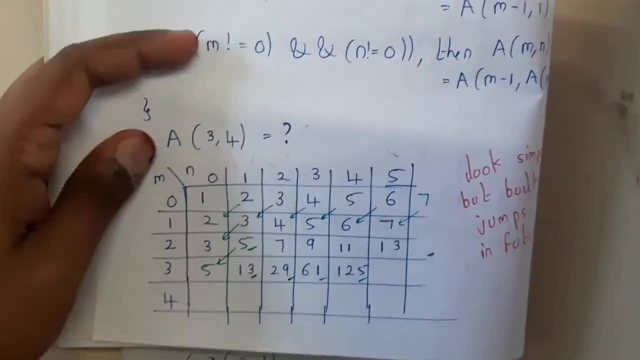 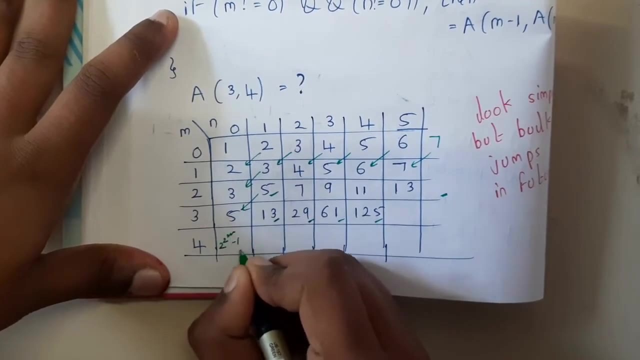 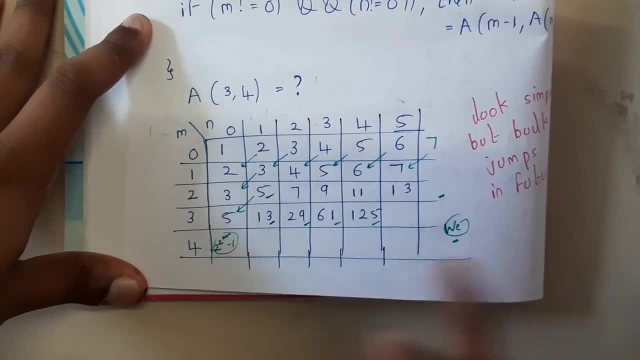 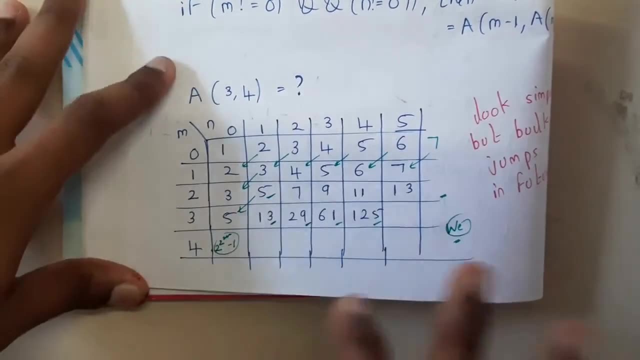 the image, guys. okay, anyway, in pdf i'll be trying to add that image after this concept. okay, yes, so it will be 2 power, power, power in that way. okay, yes, so this is a just a small example showcasing that all recursion functions are not that much easy as we think. okay, yes, so i hope everyone got. 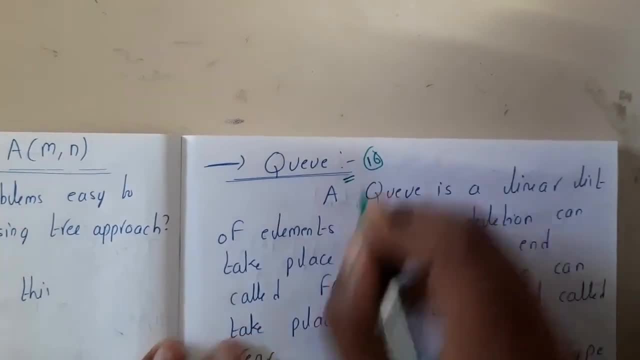 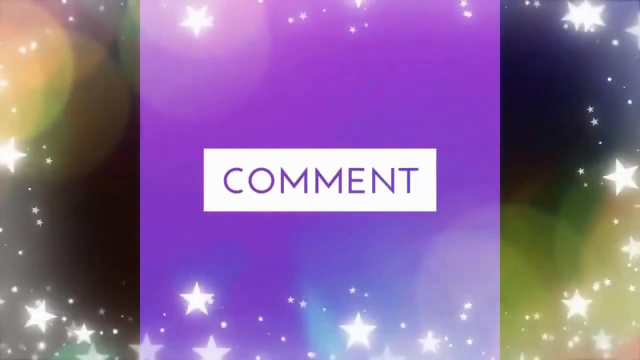 some basic idea. so in the next lecture, let us go through the concept of a qs. guys, okay, yes, so let us meet in the next lecture, thank you. thanks for watching, like, share and subscribe for more awesome videos like this. thank you. 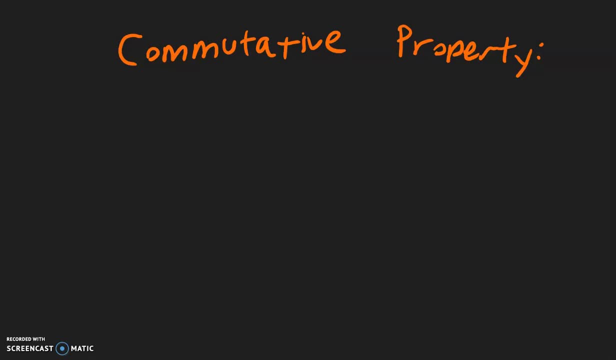 In this video we will be talking about three properties of algebra: The commutative property, the associative property and the distributive property. Commutative property. here's an example. Let's say you have 2 plus 8.. We can also write this: